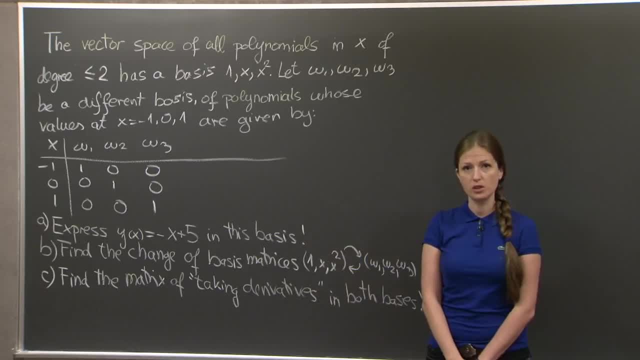 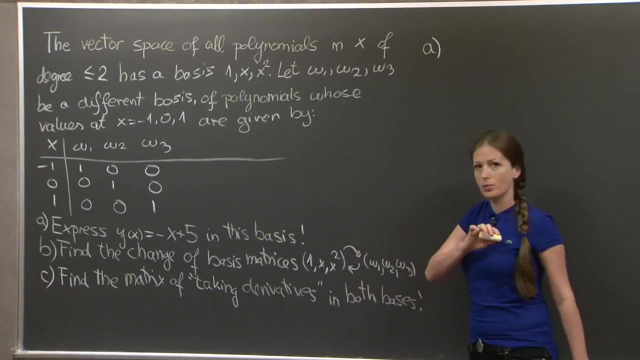 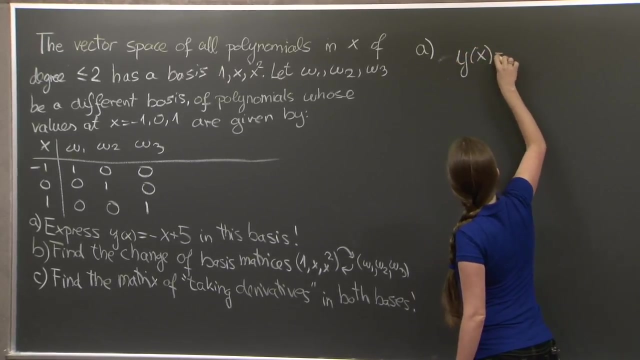 which is to try to do as much of this as possible without explicitly finding w1,, w2, and w3.. I'll let you think about the problem and then you can come back and compare your solution with mine. Hi, welcome back. So, to start with a problem A, we need to find coefficients, alpha, beta. 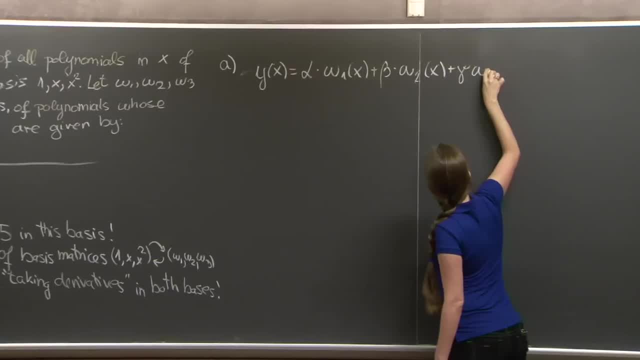 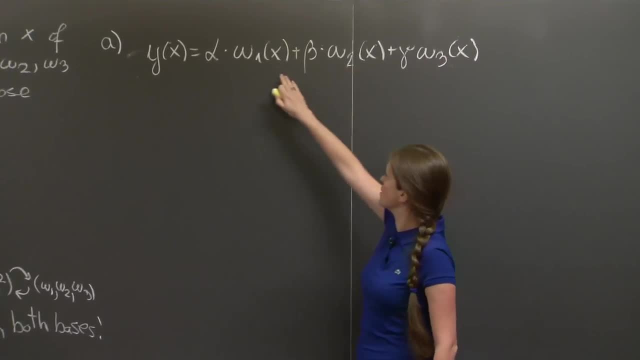 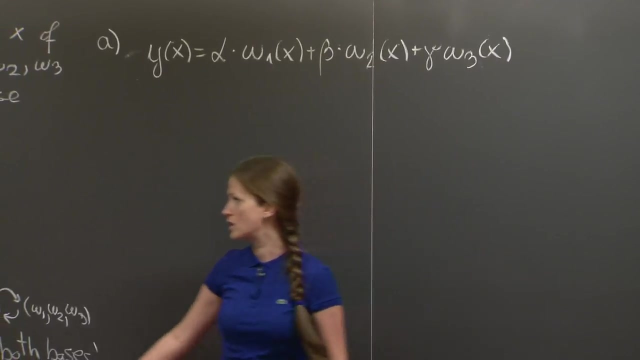 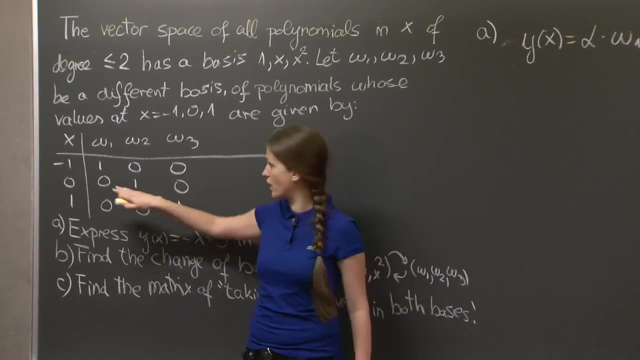 and gamma, So that y of x is expressed with this coefficient in this new basis: w1, w2, and w3.. Now one way to do that would be to look at this table of values explicitly find w1,, w2, and w3.. So a quadratic polynomial is all the information we need about it is in values. 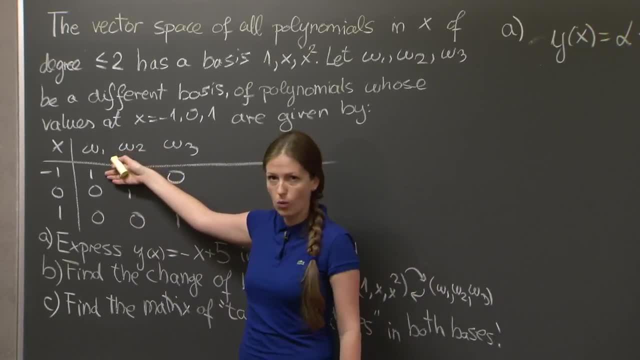 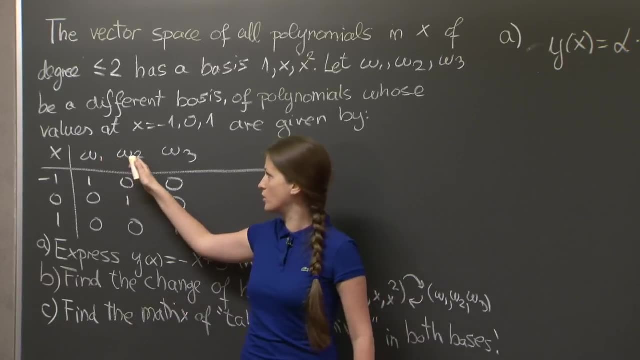 at three points. So say w1 is A1. So then we have a problem: A1 plus b, times x plus c, times x squared. Find A, b and c, Find w1,, w2, and w3 explicitly, And then go back to this system and try to find alpha. 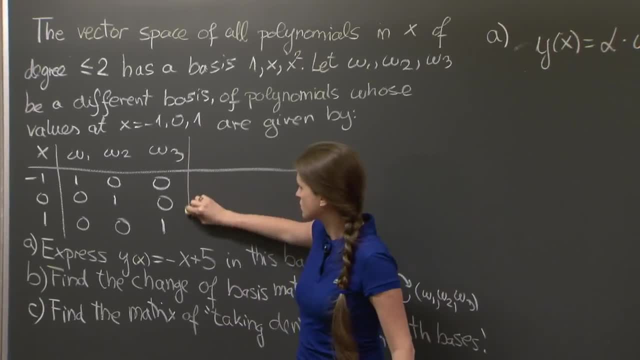 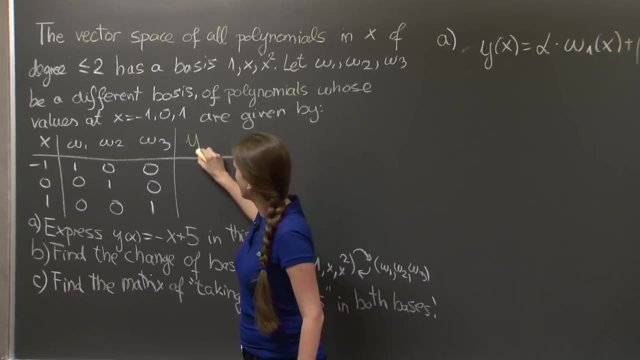 beta and gamma. However, there is a trick. Let's try to see if we can do it without finding w1, w2, and w3 explicitly. So let me try to see what are the values of y at these points. So y is minus x plus 5.. 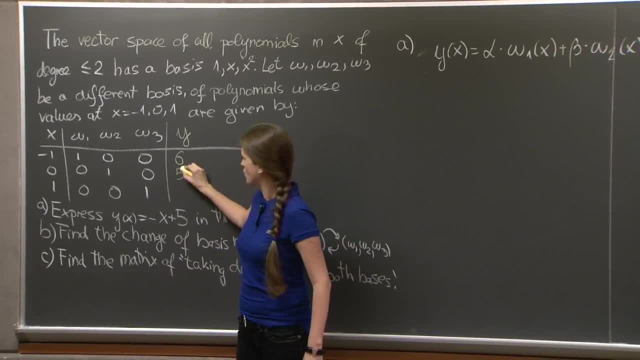 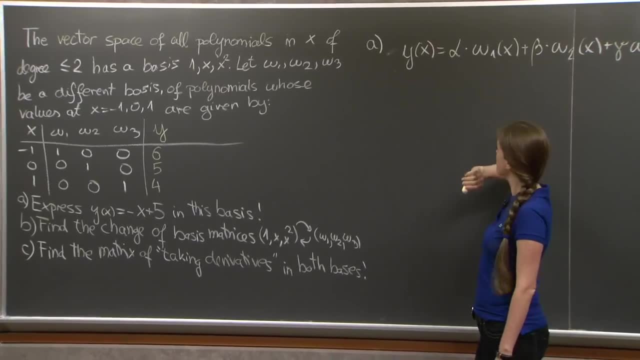 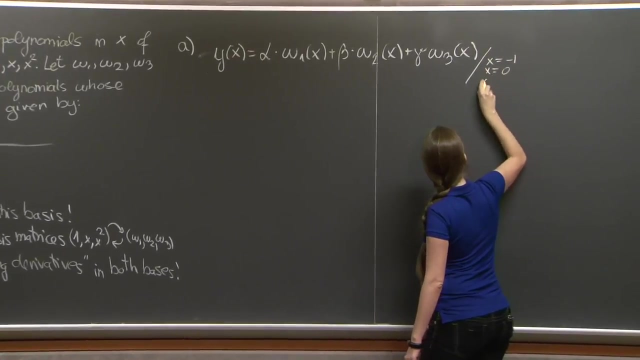 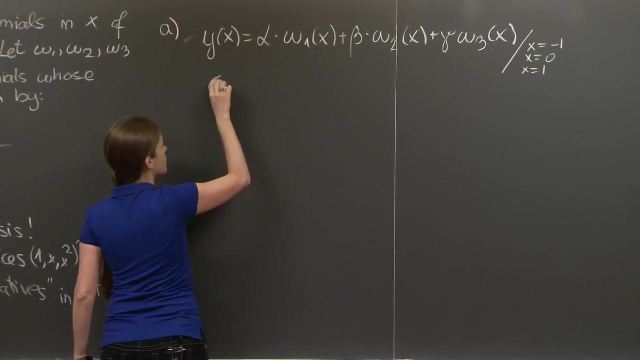 5,, so the values are 6,, 5, and 4.. And let me, instead of considering this equation, let me evaluate it at: x is minus 1,, x is 0, and x is 1.. What I get through this is that w at minus 1, actually. 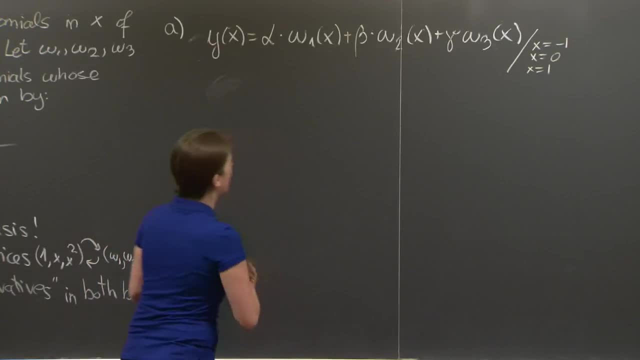 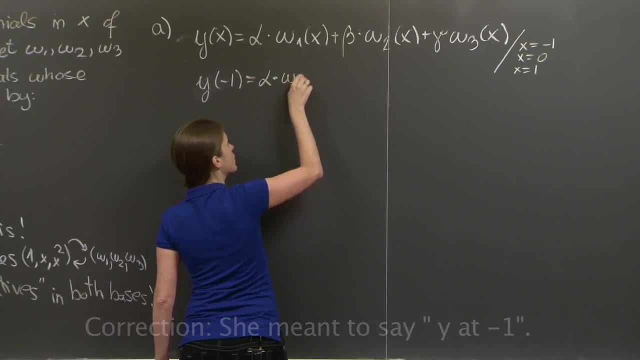 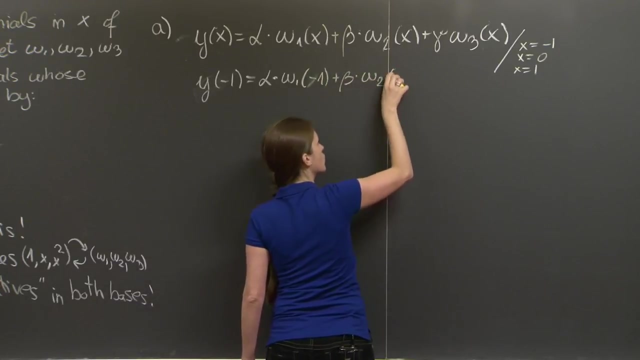 let me write this: I get that w at minus 1, which is a number equals alpha times w1 at minus 1, which is a number plus beta times w2 at minus 1, plus gamma times w3 at minus 1.. 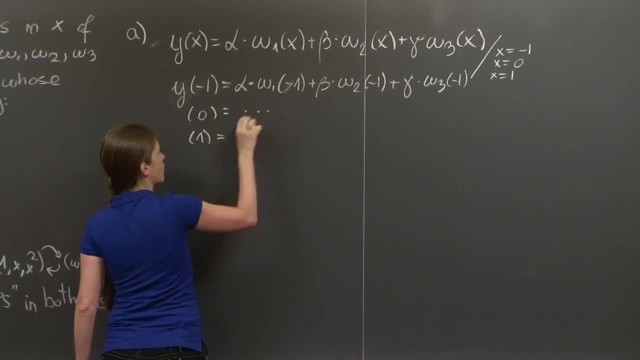 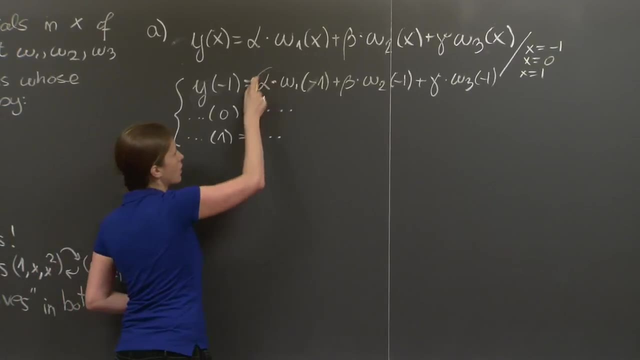 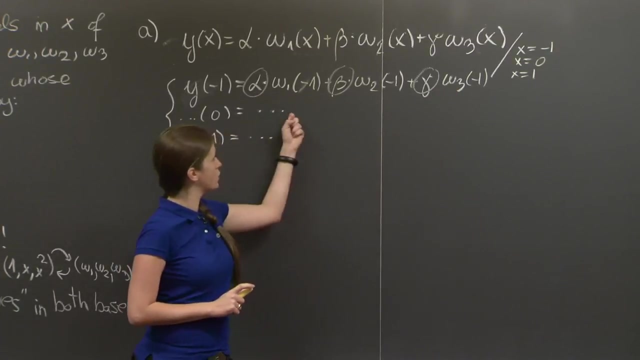 And similarly at 0.. And similarly at 0.. And similarly at 1.. And now let me think of this as a linear system that has unknowns, alpha, beta and gamma coefficients, these values here at minus 1,, 0, and 1, and the right-hand side. 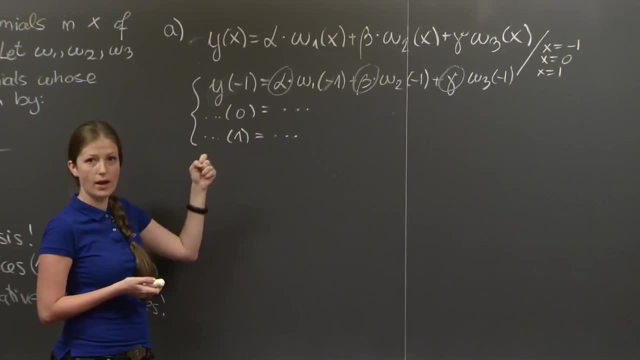 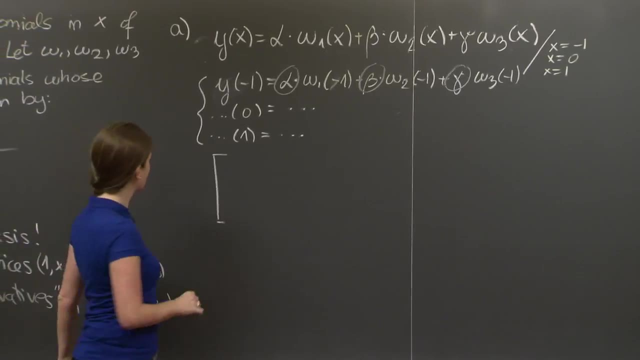 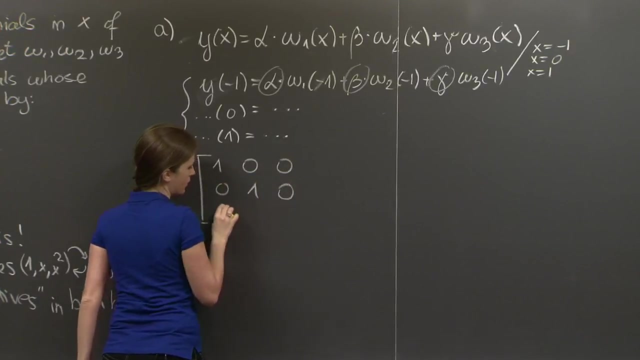 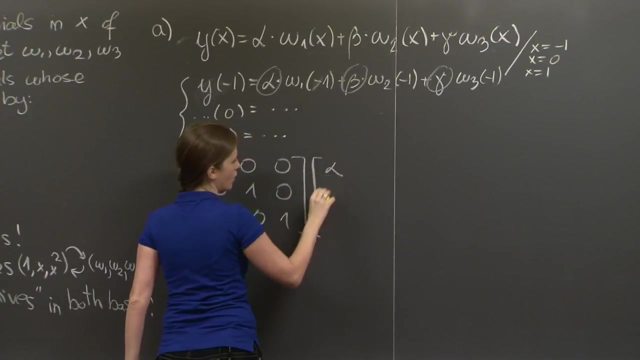 well what's written here on the left-hand side: y at minus 1,, y at 0, and y at 1.. If you write this in a matrix and read off coefficients from there, you get the following system: So this is the matrix of the system read off from here. 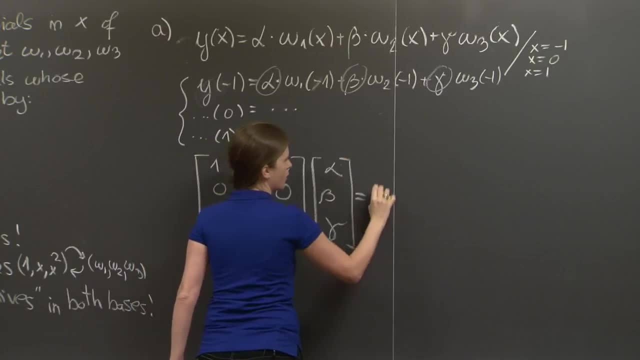 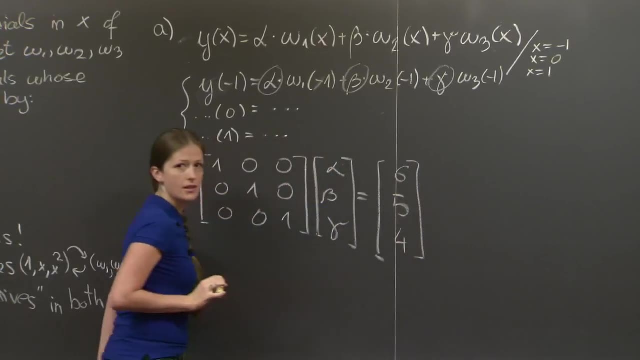 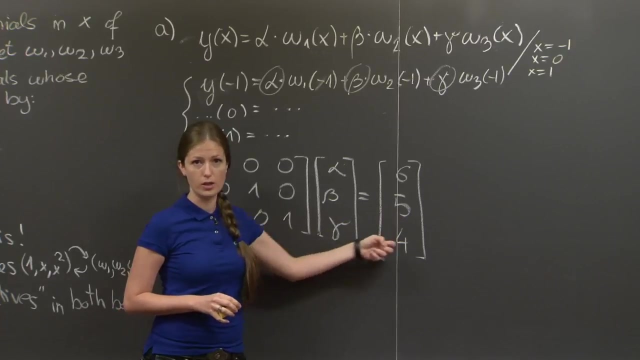 These are the unknowns and these are the values of the right-hand side, And I hope you'll agree that this is a very easy system to solve. we just get: alpha is 6,, beta is 5, and gamma is 4.. 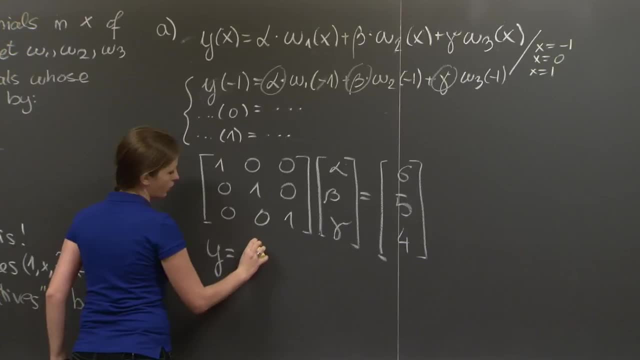 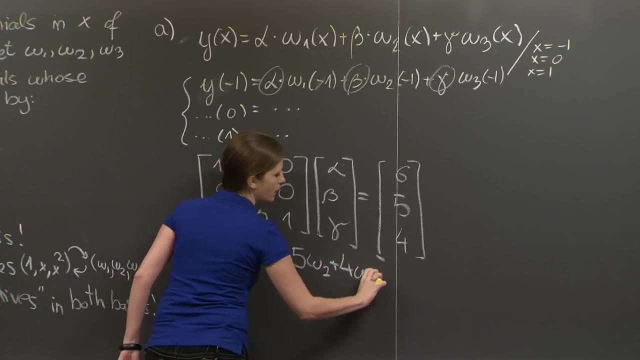 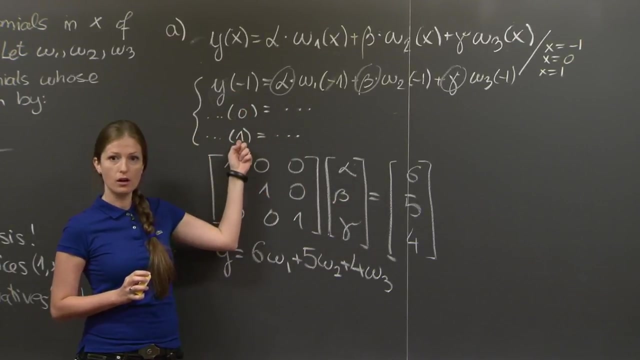 So the solution to the first part is: y equals 6w1 plus 5w2 plus 4w3.. And let's notice another thing: No matter what values we put here, this matrix is always going to stay the same. It's only the right-hand side that's going to change. 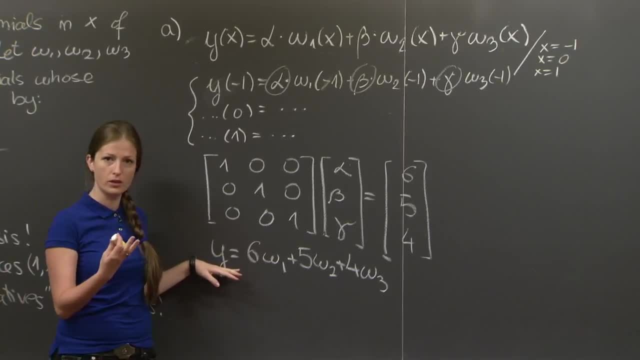 So if we're given any other polynomial now to express in a basis w1,, w2, and w3, we don't have to do the same thing, We don't have to do any thinking, We don't have to do any computations. 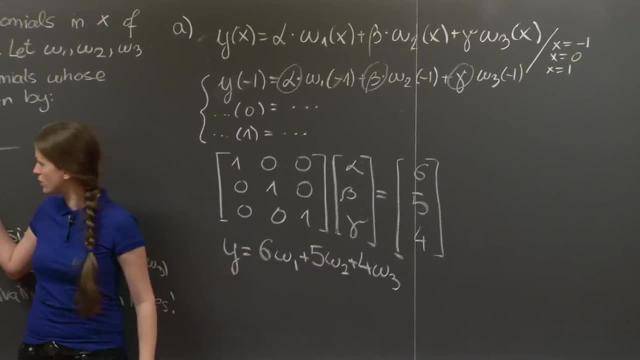 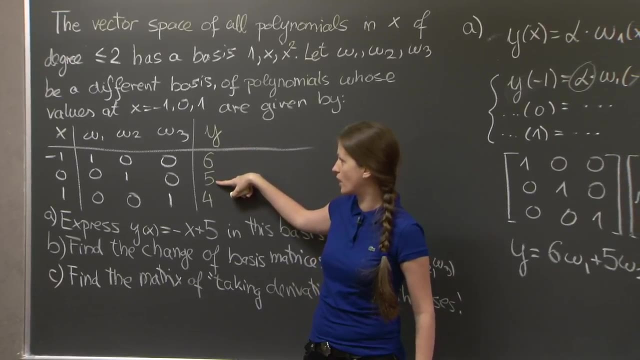 What we do is go back to our table at the beginning and just read off. let's go back to the table and just read off these values. So in this case, y is 6 times w1,, 5 times w2, and 3 times. 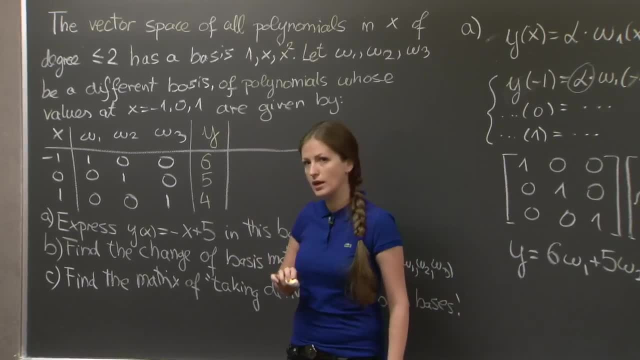 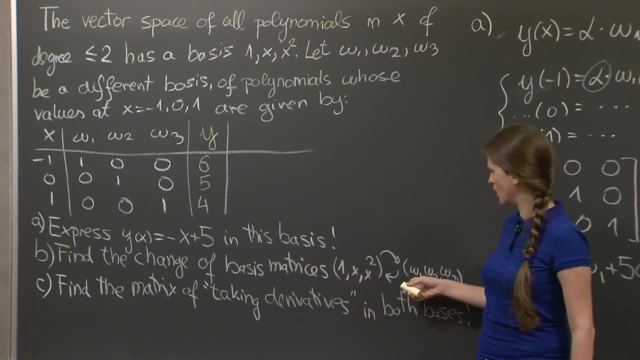 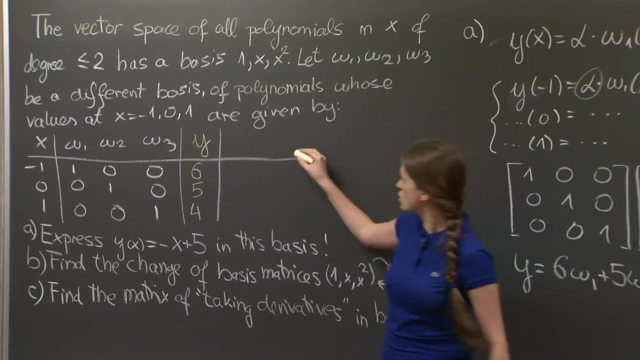 w3.. And that's already a hint to solving the b part, which is find the change of basis matrices between 1, x, x squared, and w1, w2, w3.. Change of basis matrices means expressing one basis in terms of another. 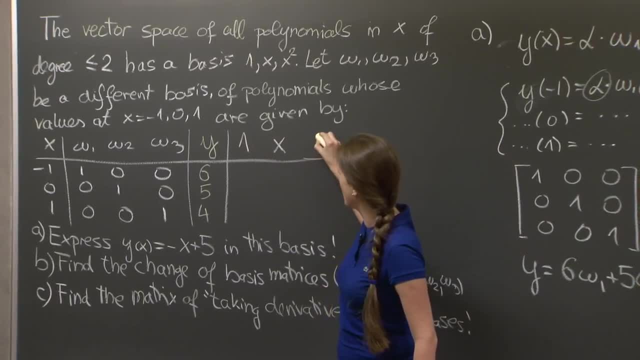 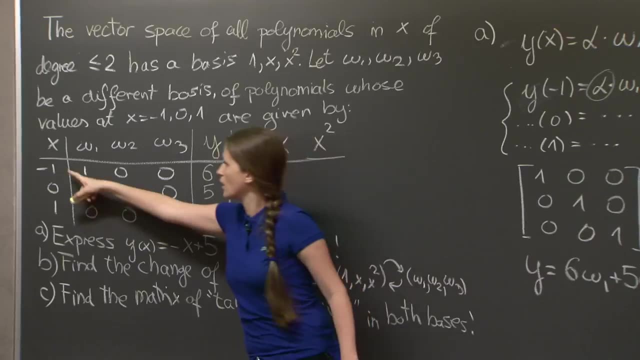 So, as a part of the problem, we will have to express 1, x and x squared in terms of w1, w2, and w3.. So let's just find their values. at these three points, 1 is a constant. 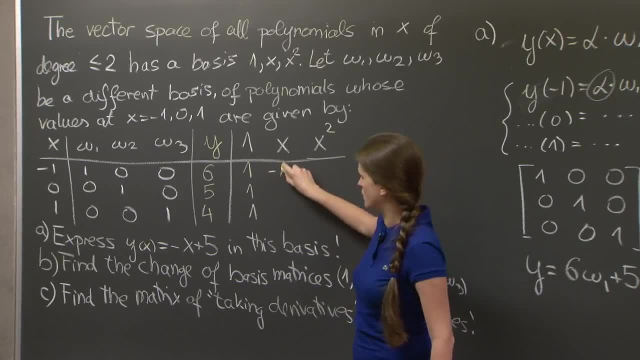 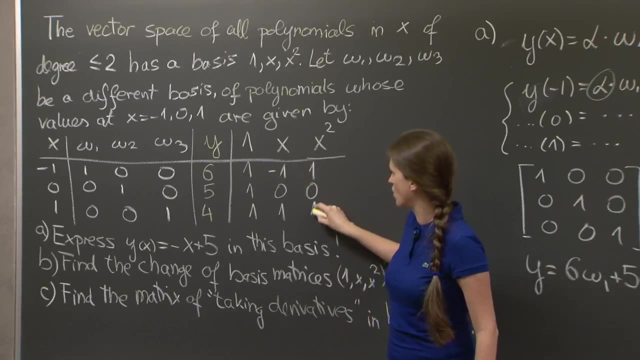 It just takes value 1 everywhere. x takes value minus 1 at minus 1,, 0 at 0, and 1 at 1.. And x squared takes values 1, 0, and 1 at minus 1,, 0, and 1.. 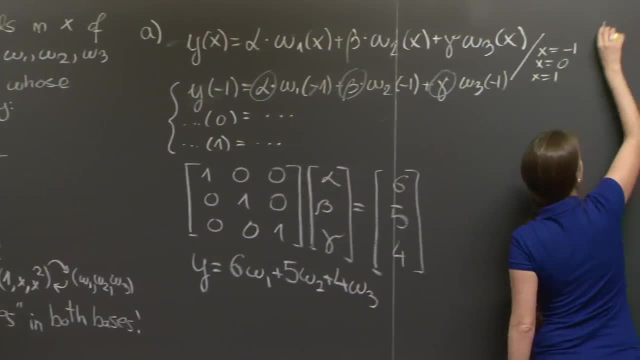 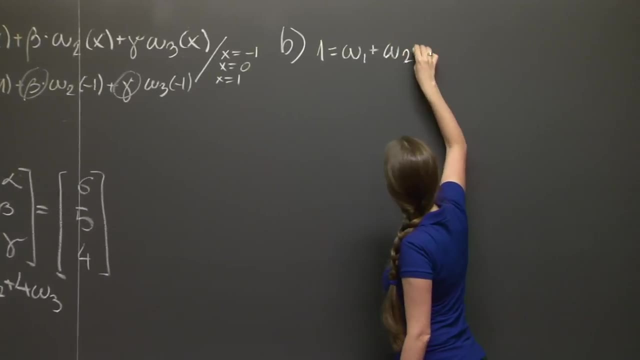 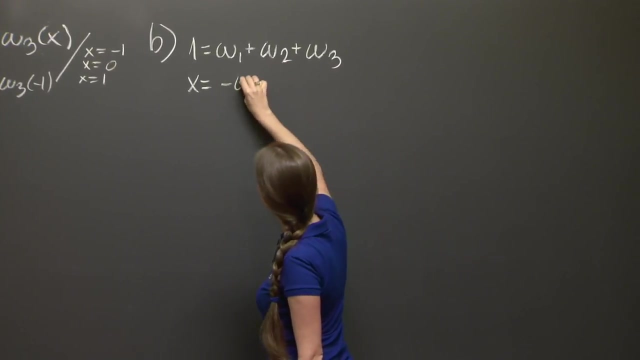 And from this we can already conclude. let's go to part b. here We can conclude that 1 equals w1 plus w2 plus w3, that x equals minus w1 plus w3, and that x squared equals w1 plus w3.. And from this we can even find the answer. Trying to solve, To solve That we can interpret from. And here I will just don't do that and get the 15.. Oh, what do you mean? Ah, I did it wrong. 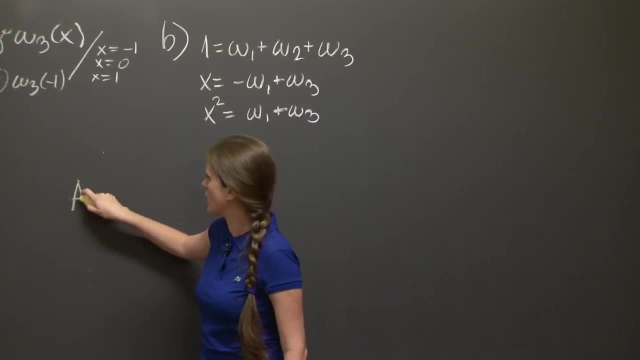 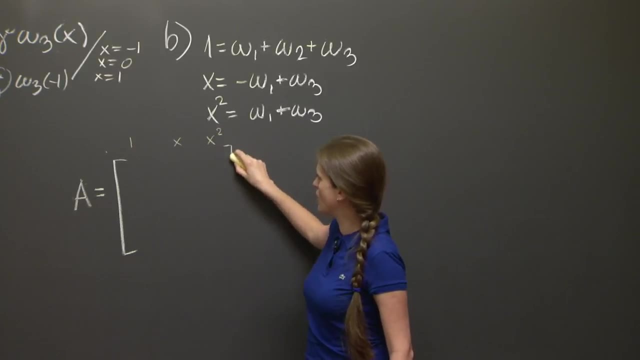 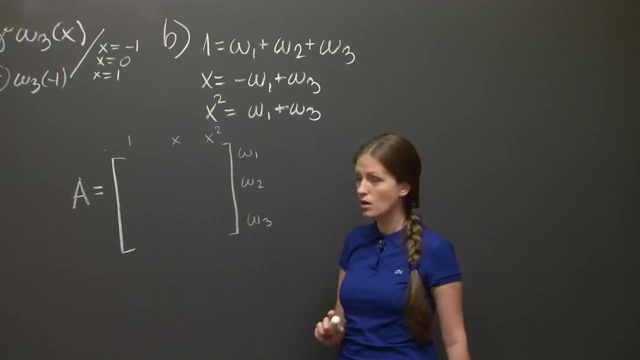 No, I did it wrong. Okay, Right, It's harder immediately write one change of basis matrix. Namely, since we know how to express 1, x and x squared in terms of w1,, w2, and w3,, we can just copy this information. 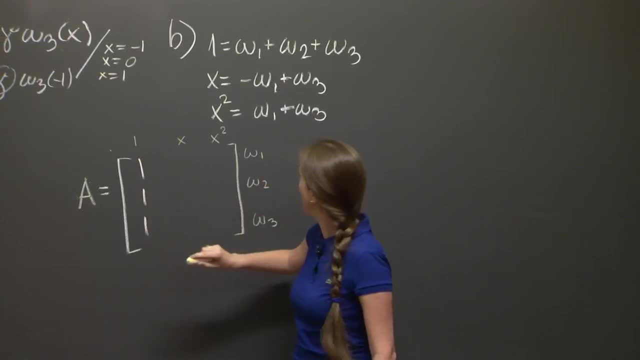 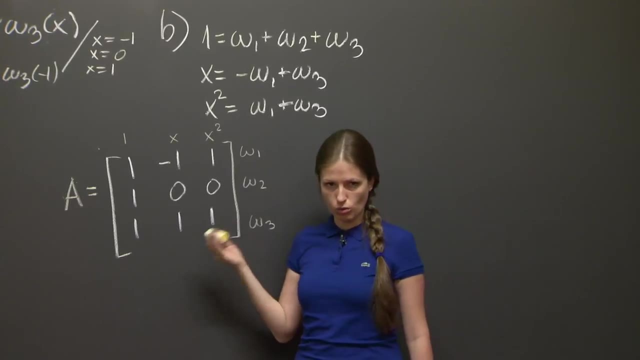 over to this matrix, getting 1, 1, 1, minus 1, 0, 1, and 1, 0, 1.. So which matrix is this? This is a matrix. so we have 1, x and x squared expressed. 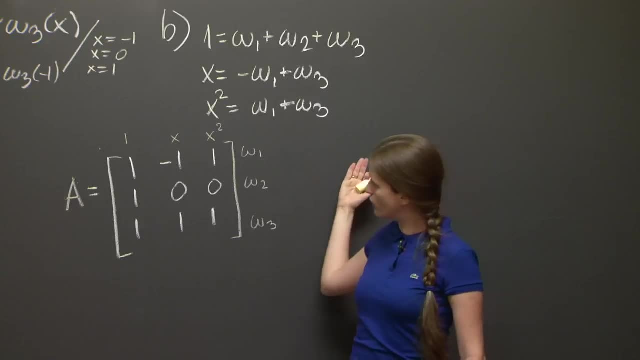 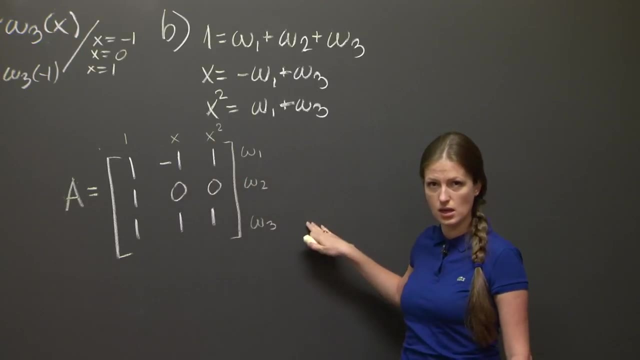 in terms of w1,, w2, and w3.. So if we feed this matrix something expressed in the basis 1, x and x squared say a, b and c, what it's going to throw out is the same polynomial expressed in this. 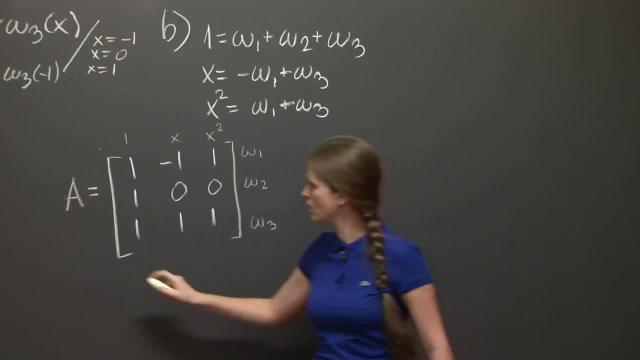 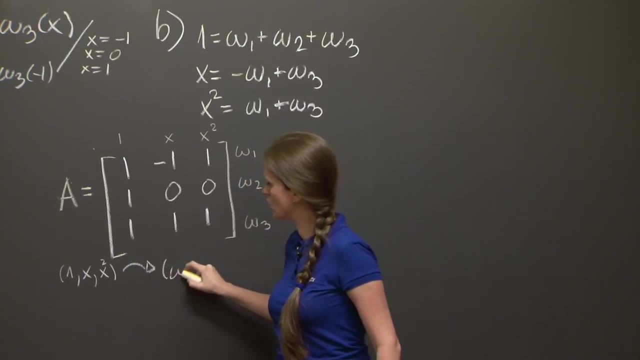 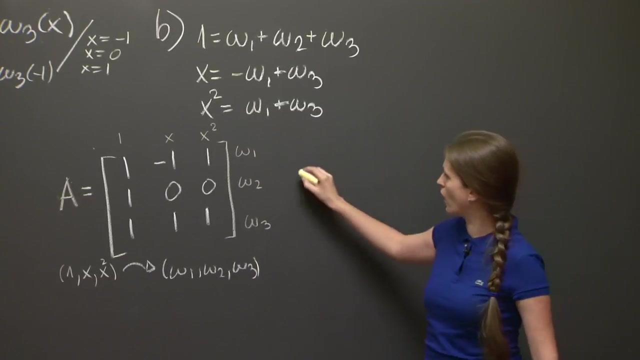 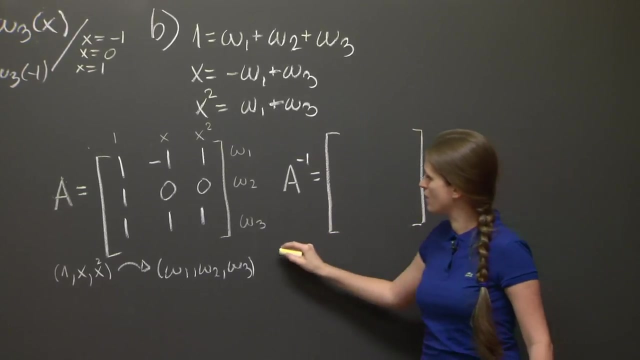 basis here: w1,, w2, and w3.. So I'm going to just write that this is a matrix of this basis change. OK, How do we get the other one? Well, very easy, We know, it's just the inverse of A. So this is going to be. 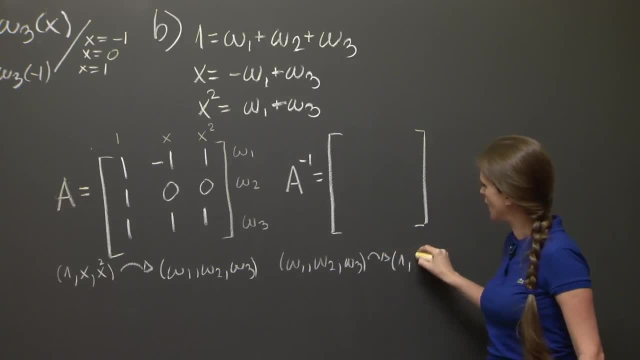 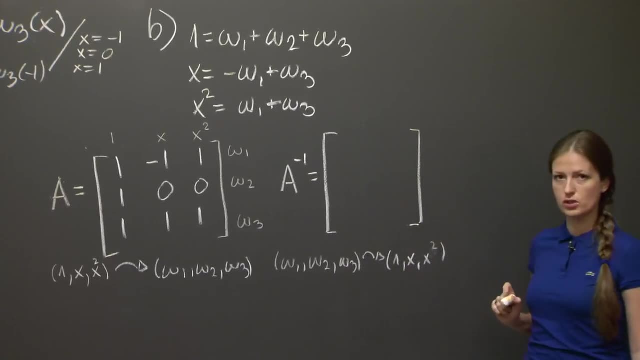 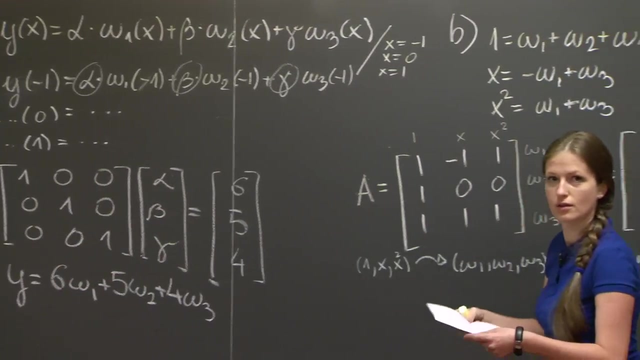 the matrix that takes something written in this basis and transfers it to this basis. I'm not going to calculate the inverse of a matrix in front of you. instead, I'm going to consult my oracle. 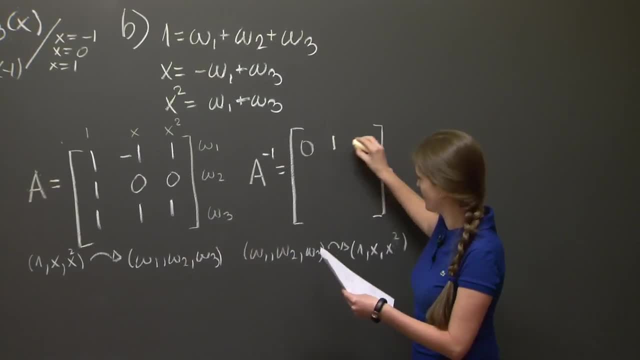 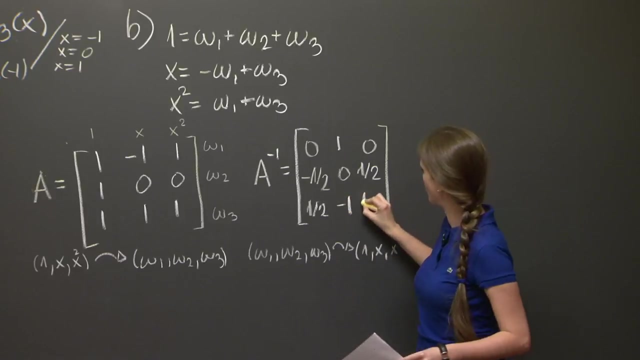 Sorry about that, And my oracle says that the inverse should be 0, 1, 0, minus 1, half, 0, 1, half and 1, half minus 1, 1, half. 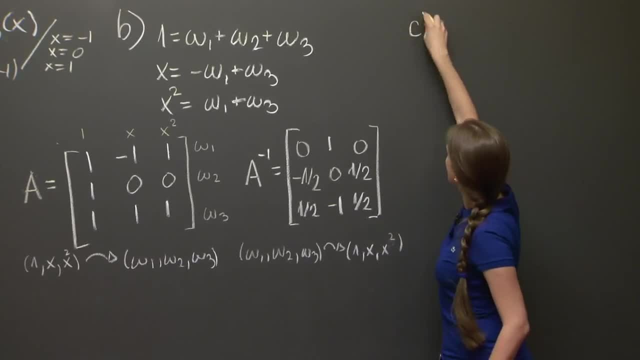 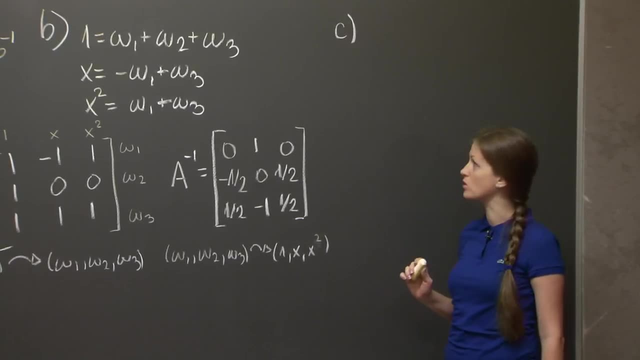 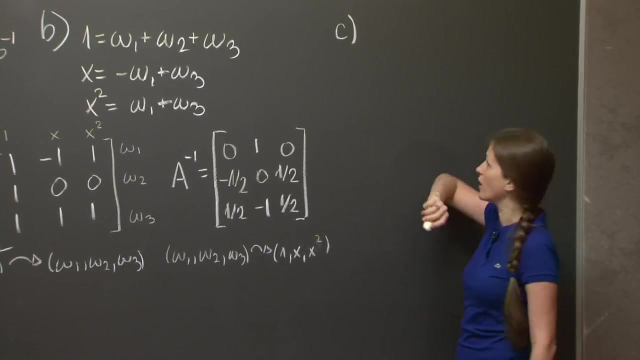 And that solves the b part. Let's go on to the c part. The c part required us to find the matrix of taking derivatives, which is a linear map on the space of polynomials in both of these bases. So let's first do the 1, x, x squared basis, because that 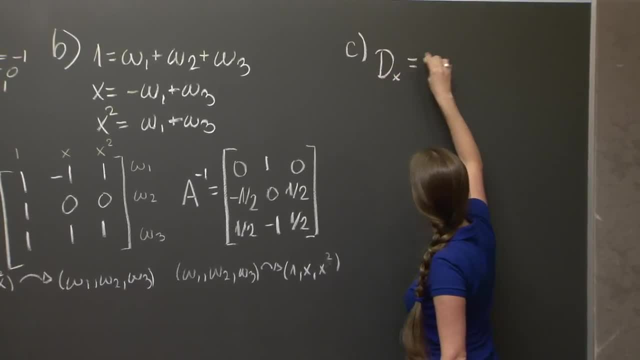 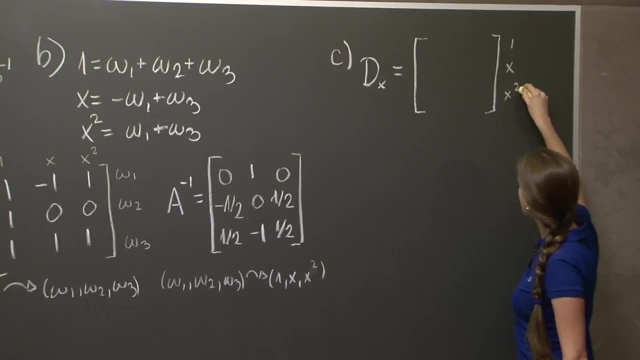 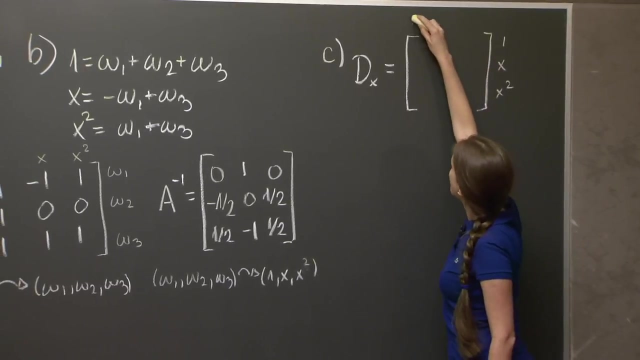 one's easier, I'm going to call it dx. So I'm going to work in basis 1, x, x squared, and what I want to explain, What I want to express, is the transformation of taking derivatives. So here I'm going to write the vector to which taking 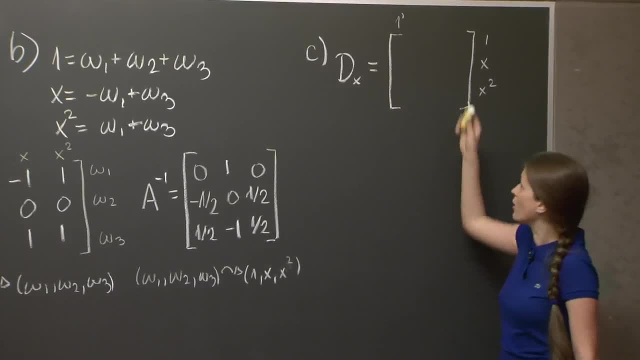 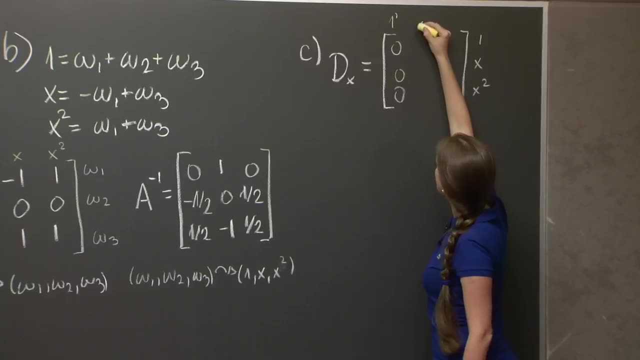 derivatives maps, the polynomial 1,, which is 0.. And that's this expressed in the basis 1, x, x squared. In the second column, I'm going to write x, prime, the vector to which dx sends the vector x, and that's equal to. 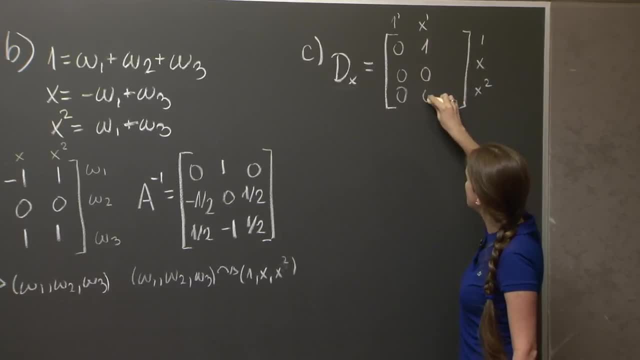 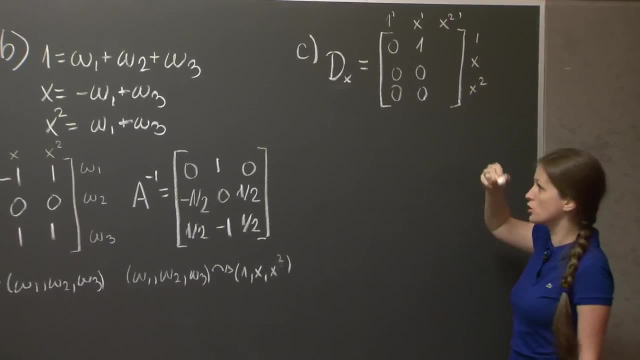 1, which, expressed in this, The vector to which dx is expressed in this basis, is 1, 0, 0.. And here I'm going to write x squared prime, which is 2x, which, expressed in this basis, is just this. 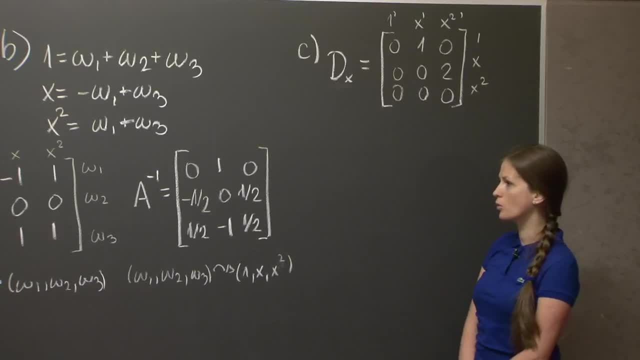 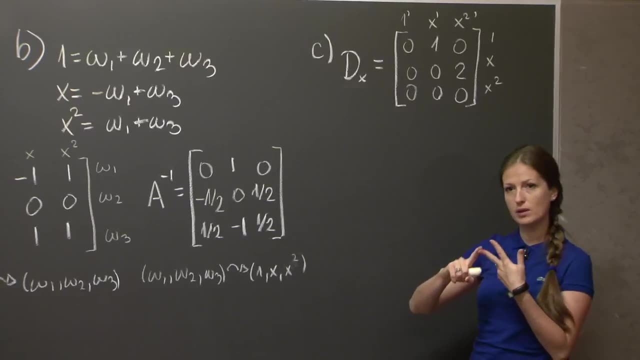 OK, That one was easy. For the other one, well, we could calculate w1, w2, w3 explicitly, take their derivatives, go back to the table and try to find and repeat the procedure that we did already. So express the derivative. 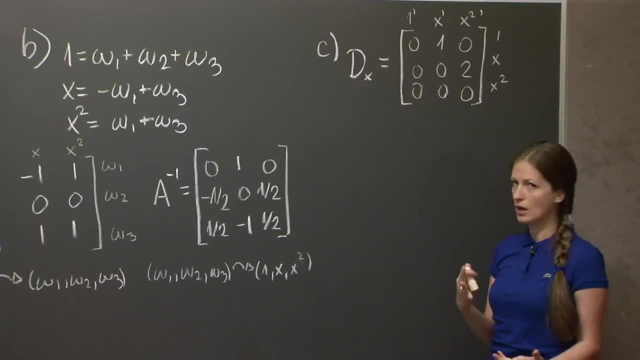 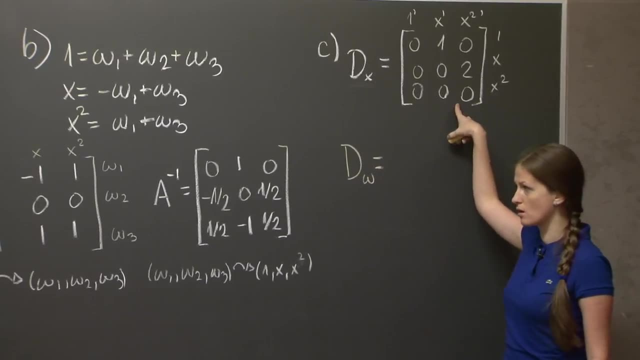 So express the derivative, So express the derivative. So we're expressing these derivatives in terms of w1, w2, w3, and that's a lot of work, But we pretty much already did most of this work, So we know how to take derivatives in this basis and 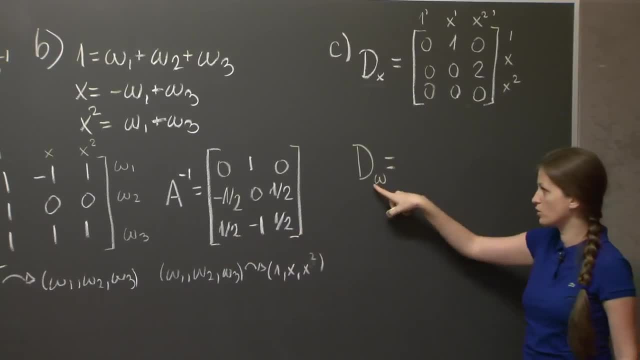 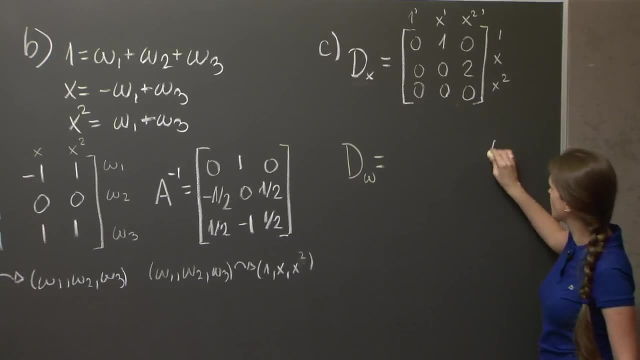 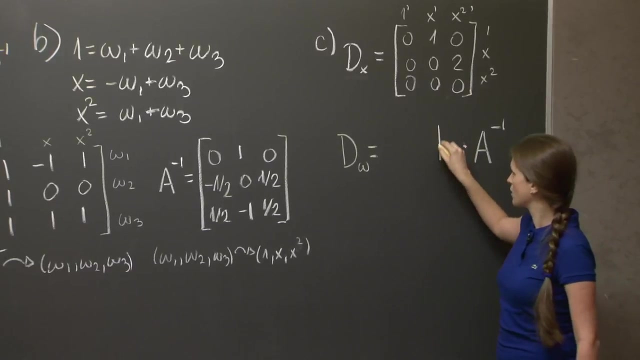 we know how to go between these two bases. So if we want to take a derivative of something written in the basis w1, w2, w3,, well, let's first write this something in basis 1, x, x, squared.